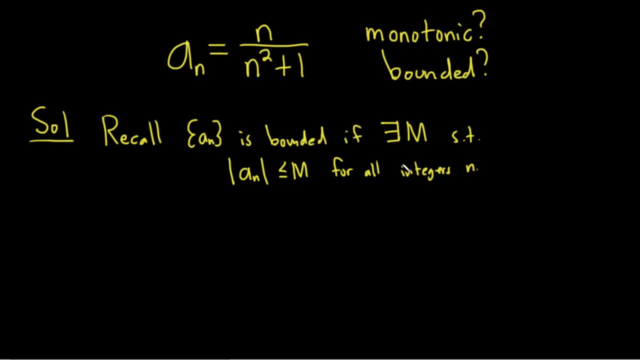 me take this opportunity to show you the way to do this, with the definition of what it means for a sequence to be bounded Typically. when you learn this in calculus, you might not be doing it this way, so it's just a fun way to do it. So we just have to find an m and create this inequality here. 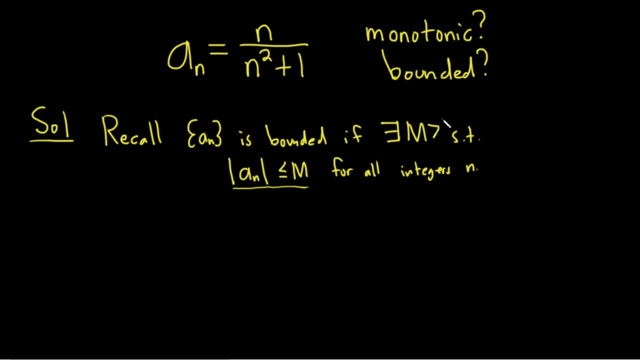 If you like, you can specify that m is positive. That's typically something people do, Okay, so let's go ahead and take the absolute value of a sub n, and that's equal to the absolute value of n over n squared plus 1.. 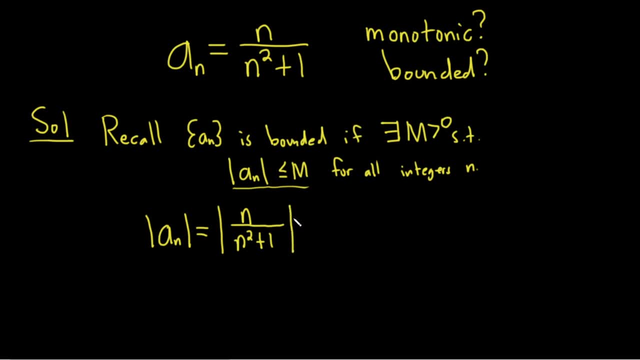 And this is going to show you a technique that's actually really useful in proofwriting. so that's another reason I wanted to do it this way. It's worth learning some extra stuff. So we want to make this less than or equal to something. So, whenever you have a denominator, 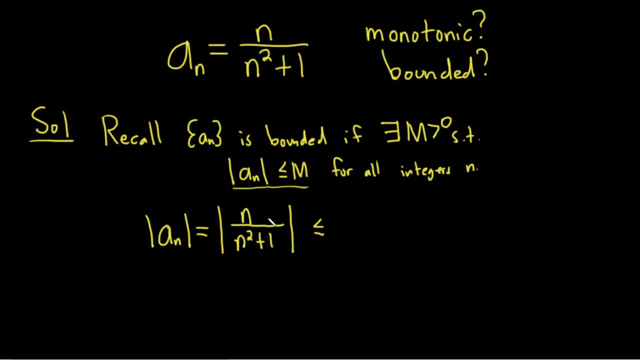 like this in order to make this fraction smaller than whatever I write here. I can just do this. I can drop the 1.. And the reason I can do that- okay, the reason I can drop that positive number- is because n squared plus 1 is equal to 1 over n squared plus 1.. 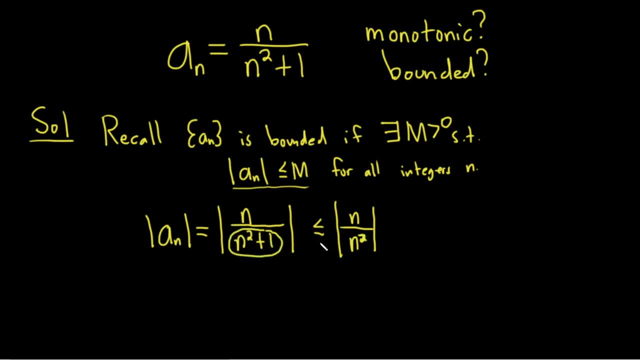 Okay, so this is going to show you a technique that's actually really useful in proofwriting, so that's another reason I wanted to do it this way. It's worth learning some extra stuff. So remember: n squared plus 1 is bigger than n squared, so it makes the fraction over here. 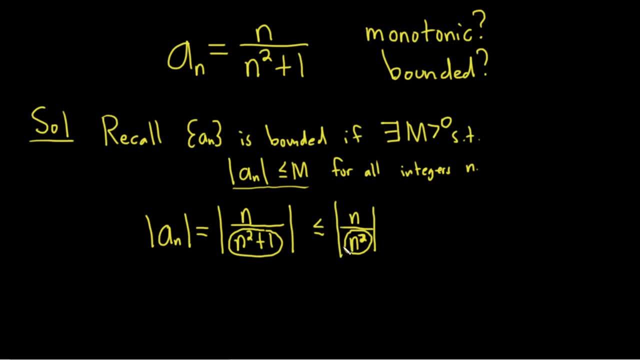 on the left smaller than the fraction over here on the right. It's actually a smaller number because the bottom part is bigger, right? Just think simple. Think like: 1 over 5 is smaller than 1 over 4, and 5 is a bigger number than 4, right? So the same thing is. 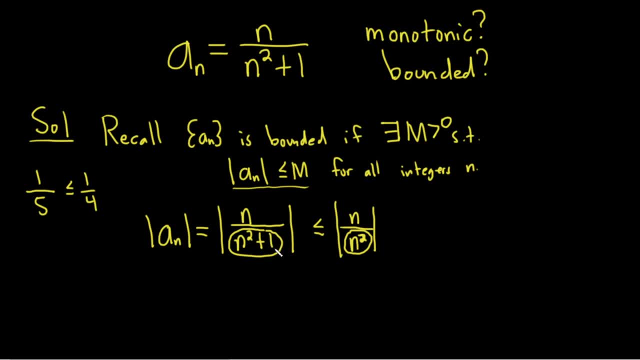 happening here and it's a little more clear because we're adding that 1, so it's certainly bigger than n squared. and all of these are positive integers, so we can drop the absolute value and at the same time now let's just go ahead and cancel one of the n's, so we're left with one over. 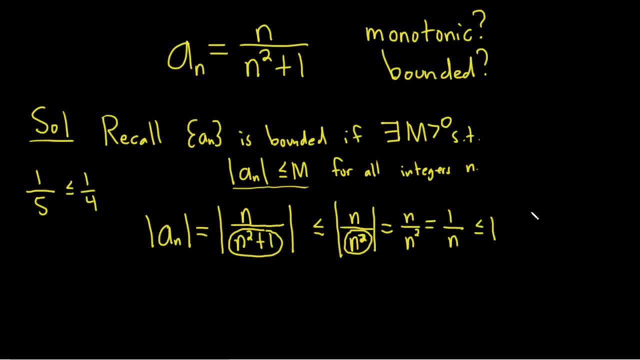 n, and this is certainly less than or equal to one, and that's because n is greater than or equal to one right. so the smallest it can be is one, and if you were to divide both sides of this inequality by n, you would end up with something like this, which you can then read backwards: one over n. 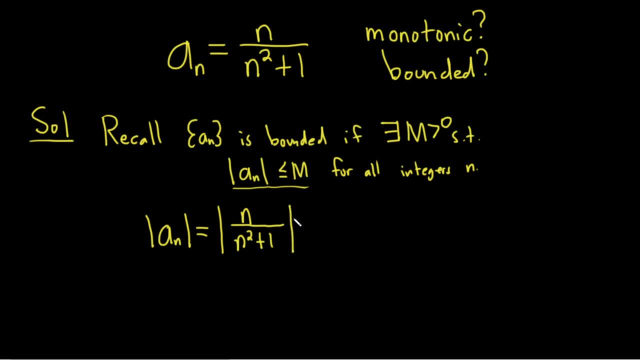 And this is going to show you a technique that's actually really useful in proofwriting. so that's another reason I wanted to do it this way. It's worth learning some extra stuff. So we want to make this less than or equal to something. So, whenever you have a denominator, 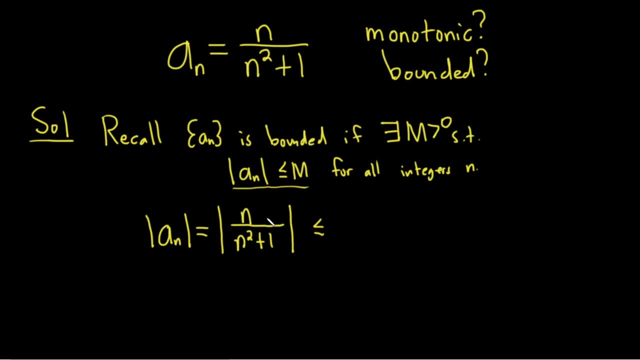 like this in order to make this fraction smaller than whatever I write here. I can just do this. I can drop the 1.. And the reason I can do that- okay, the reason I can drop that positive number- is because n squared plus 1 is equal to 1 over n squared plus 1.. 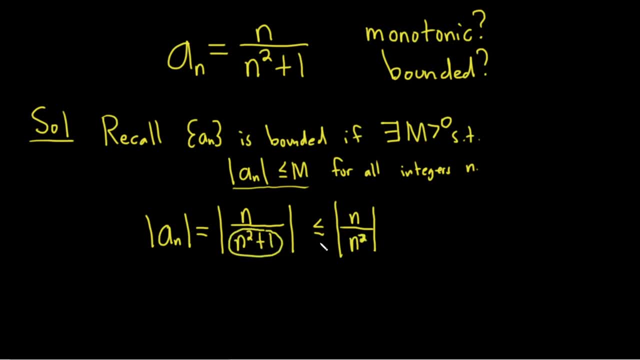 So I can just do this. I can drop the 1.. And the reason I can do that- okay, the reason I can drop that positive number- is because n squared plus 1 is equal to 1 over. n squared plus 1 is bigger than n squared, So it makes the fraction over here on the left smaller. 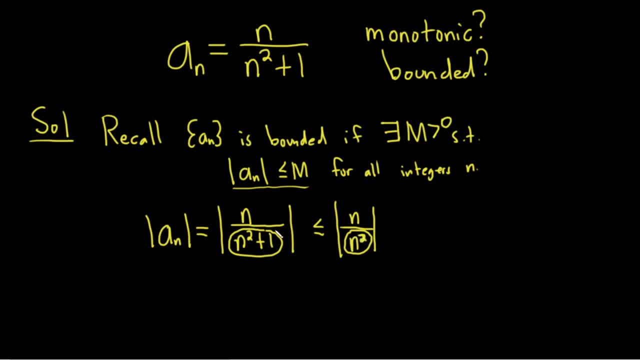 than the fraction over here on the right. right It's actually a smaller number because the bottom part is bigger, right? Just think simple. Think like: 1 over 5 is smaller than 1 over 4.. And 5 is a bigger number than 4,, right? So the same thing is happening here. 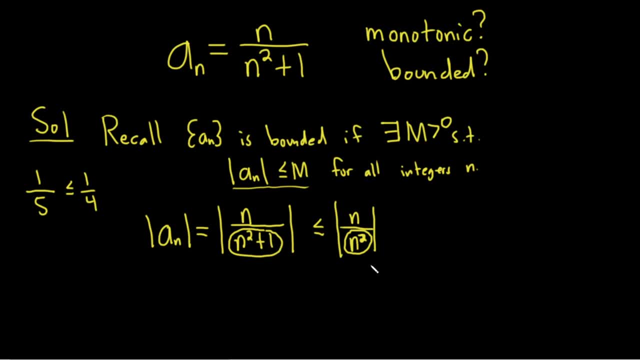 And it's a little more clear because we're adding that 1.. So it's certainly bigger than n squared. And all of these are positive integers, so we can drop the absolute value And at the same time, now let's just go ahead and cancel one of the n's, So we're left with 1 over. 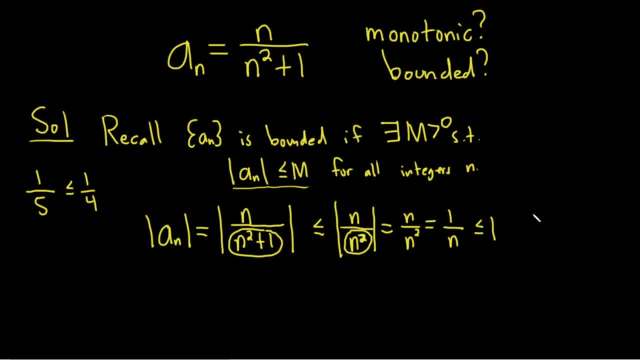 n, And this is certainly less than or equal to 1.. And that's because n is greater than or equal to 1, right, So the smallest it can be is 1.. And if you were to divide both sides of this inequality by n, you would end up with something like this, which you can then: 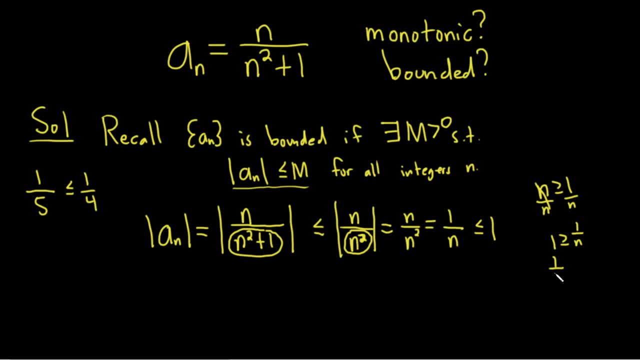 read backwards: 1 over n less than or equal to 1.. Boom, Really important type of thinking if you ever take some advanced calculus, So note so. so a sub n is less than or equal to 1. And that's true for all integers n, I should say. I should really say positive. 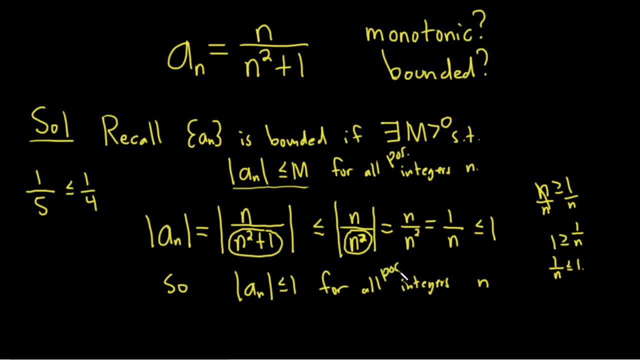 integers n right, Because you know we're assuming the sequence here starts at 1.. So all right, So it's bounded. So thus it is bounded, So to show it's monotonic. what we're going to do is, again, we're going to take a really 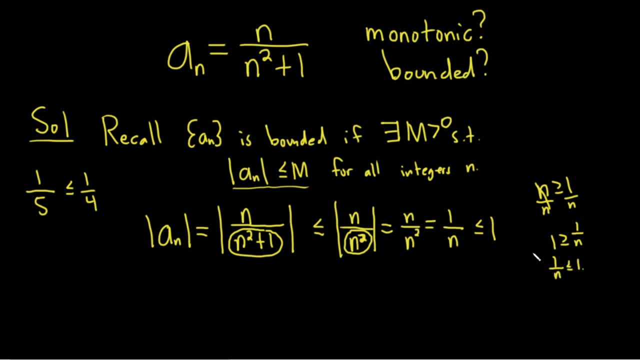 less than or equal to one. boom, really important type of thinking. if you ever take some advanced calculus, so note so. so a sub n is less than or equal to one, and that's true for all integers n, i should say. i should really say positive integers n. right, because 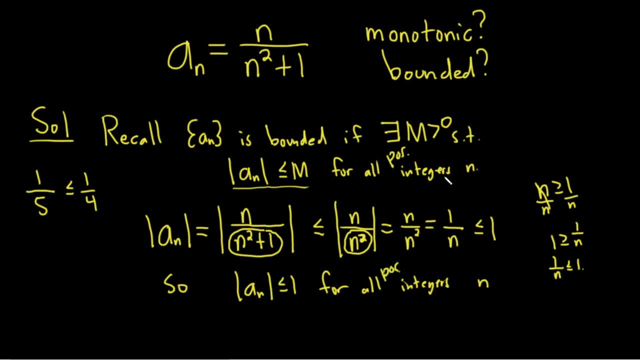 you know, we're assuming the sequence here starts at one. so all right, so that's. so it's bounded. so thus it is bounded, so to show it's monotonic. um, what we're going to do is, again, we're going to take a really rigorous approach here. we're going to do the following, so i'm just going to let 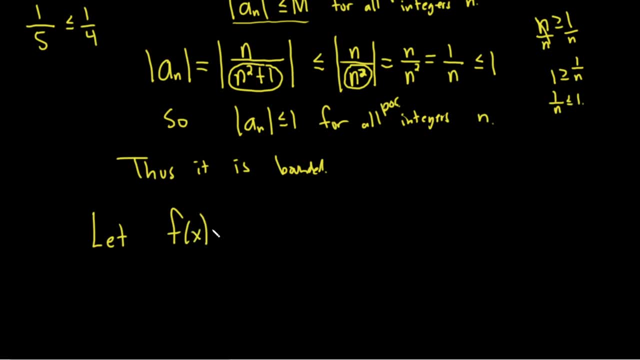 f of x be equal to x over x squared plus one. so we're going to do the following. so i'm just going to let f of x be equal to x over x squared plus one. so we're thinking of our sequence, which was a sub n n over n squared plus one as a function of x, and the reason 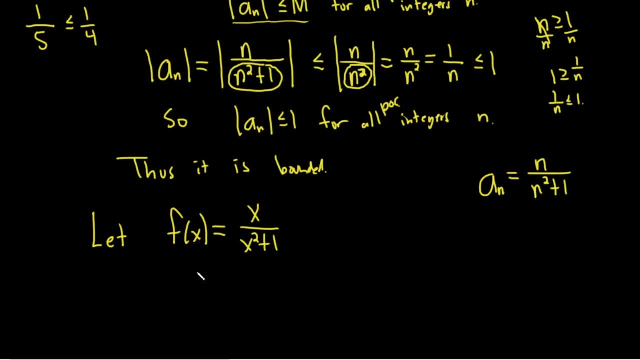 we're doing that is because we're going to take the derivative and see if it's positive or negative. remember, if the derivative is positive on an interval, the function is increasing on an interval. if the derivative is negative on an interval, the function is decreasing on an. 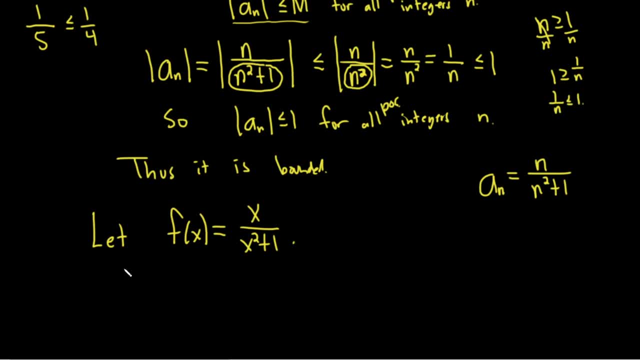 interval. so let's go ahead and take the derivative and see what comes from that and just recall that there is a formula for the derivative of a quotient. i hate to use the same variable but i will. so if you have f over g and you're taking the derivative, you can think of f as your top function and g as your. 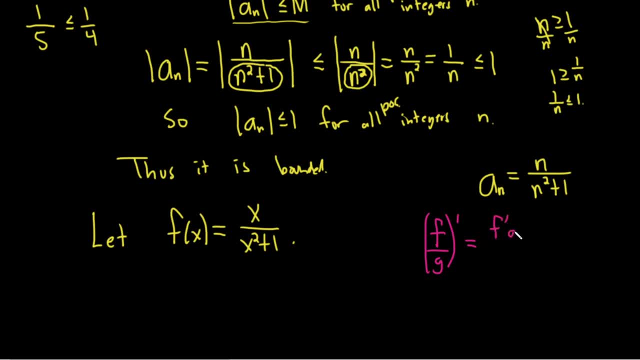 bottom function. it's the derivative of the top times the bottom minus the top times the derivative of the bottom all over the bottom, one squared. so here x is our top and x squared plus one is our bottom function. so it's the derivative of the top times the bottom. 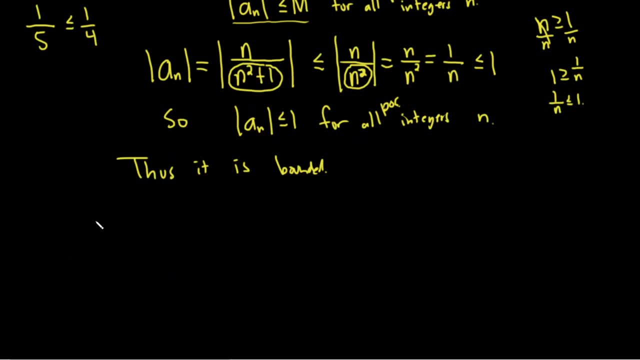 rigorous approach here. We're going to do the following. So I'm just going to let f of x be equal to x over x squared plus 1.. So we're thinking of our sequence, which was a sub n n over n squared plus 1.. 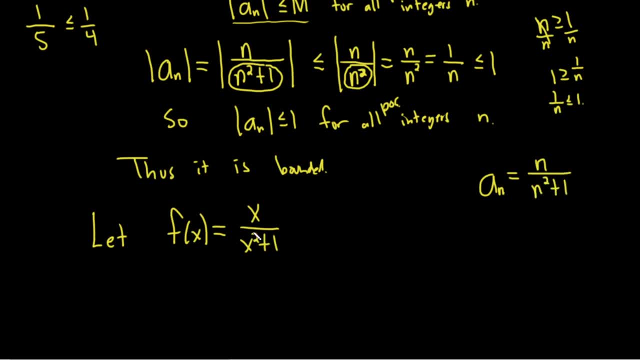 As a function of x, And the reason we're doing that is because we're going to take the derivative and see if it's positive or negative. Remember, if the derivative is positive on an interval, the function is increasing on an interval. If the derivative is negative on an interval, 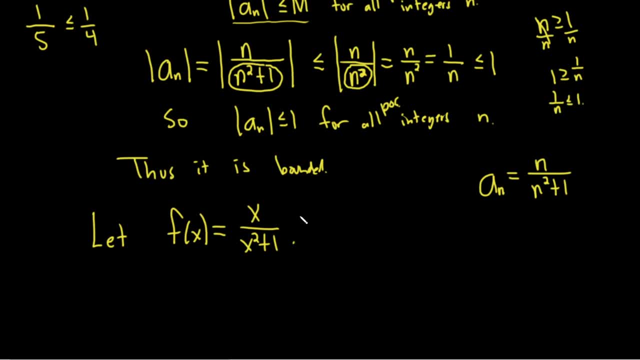 the function is decreasing on an interval. So let's go ahead and take the derivative and see what comes from that And just recall that there is a formula for the derivative of a quotient: 1 over n, less than or equal to 1.. 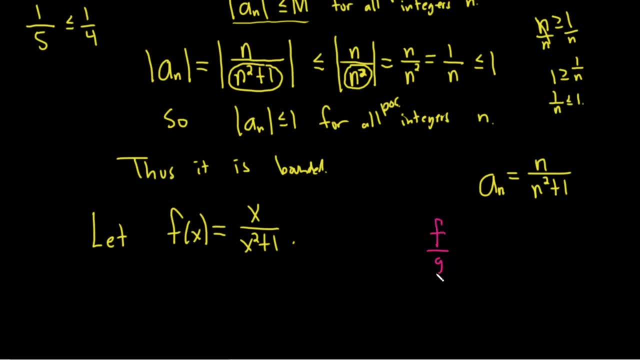 I hate to use the same variable but I will. So if you have f over g and you're taking the derivative, you can think of f as your top function and g as your bottom function. It's the derivative of the top times the bottom minus the top times, the derivative of the. 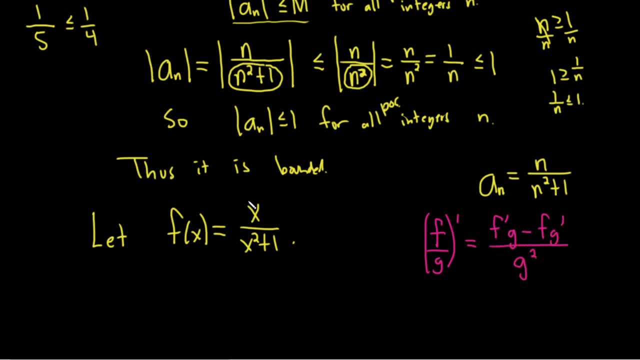 bottom, all over the bottom, 1 squared. So here x is our top and x squared plus 1 is our bottom function. So it's the derivative of the top times the derivative of the bottom. So if you have n less than or equal to 1, you can take the derivative of the bottom. 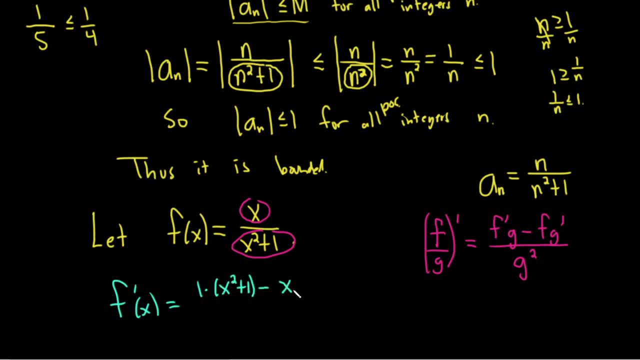 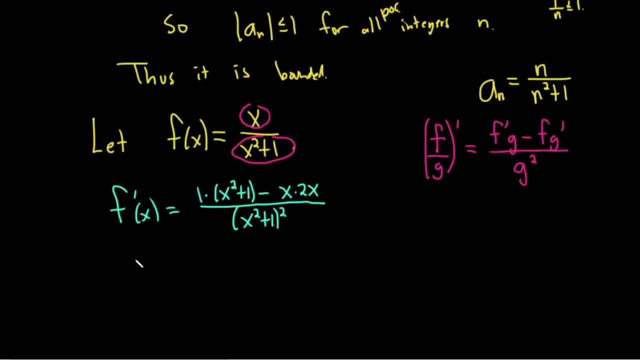 and you're taking the derivative of the bottom all over. the derivative of the bottom minus the top times the derivative of the bottom, which is simply 2x, using the power rule all over the derivative of the bottom, 1 being squared Just some quick quotient rule action. So this is f prime of x. So the 1 times this is just. 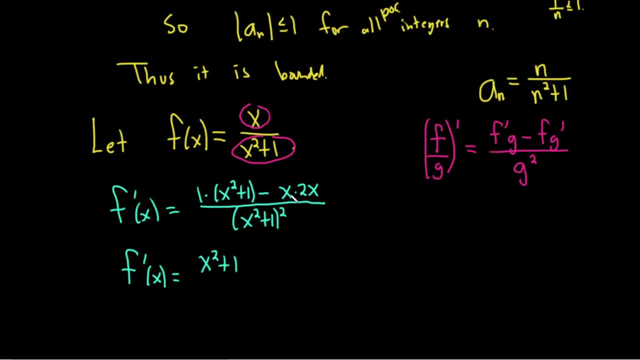 going to be x squared plus 1.. No big deal there. And then here, x times 2x is minus the 2x squared. And on the bottom, here you have. and this is just one way to do it. There's other ways. 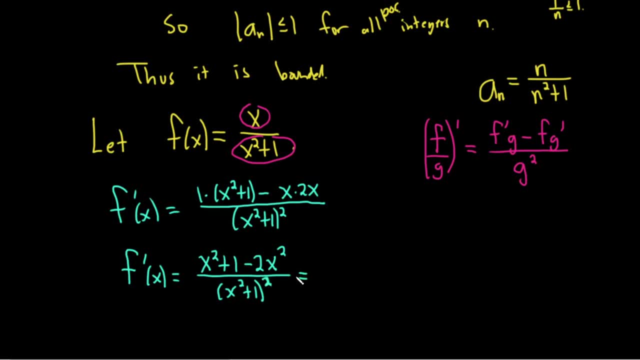 to do it right. This is just I figured. let me just take this video as an opportunity to show you how to do it this way. So x squared minus 2x squared is negative, x squared right, Because there's really a 1 here. So 1 minus 2 is negative 1, and then plus 1.. And this here is x squared. 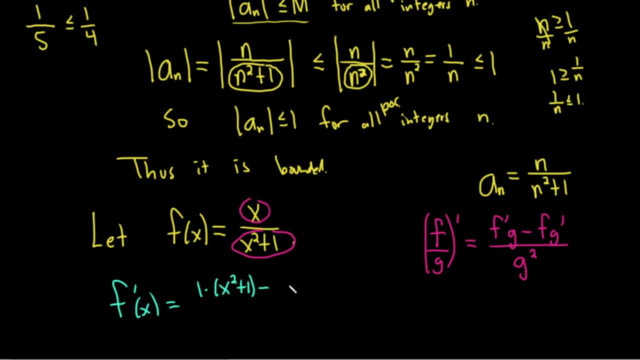 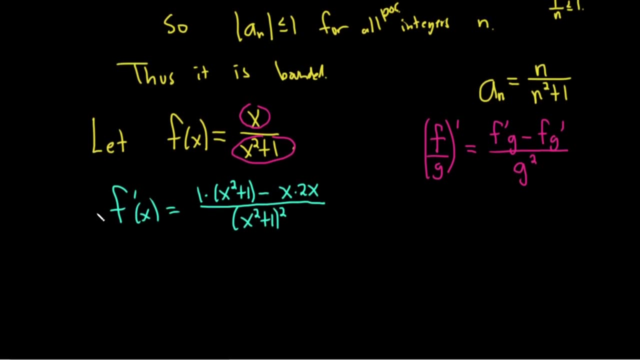 minus the top times the derivative of the bottom, which is simply 2x, using the power rule all over the derivative of the bottom one being squared, just some quick quotient rule action. so this is f prime of x. so the one times this is just going to be. 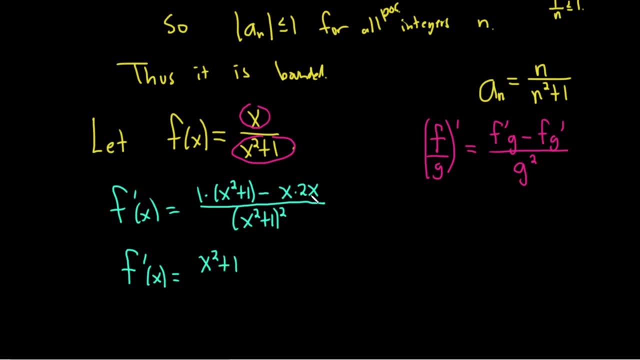 x squared and the derivative of the bottom one is going to be x squared plus one. no big deal there. and then here, x times 2x is minus 2x squared, and on the bottom, here you have. and this is just one way to do it. there's other ways to do it right. this is just i figured. 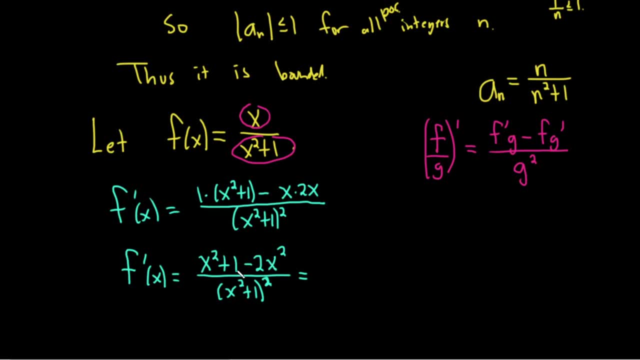 let me just take this video as an opportunity to show you how to do it this way. so x squared minus 2x squared is negative, x squared right, because there's really a one here. so one minus two is negative one, and then plus one, and this here is x squared plus one squared. 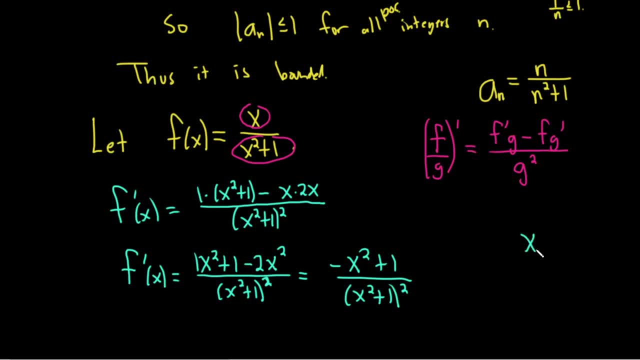 and in all of this, we have to remember, um, that x is greater than or equal to one. okay, that's really important. let's write it like this: one minus x squared over, x squared plus one squared. this is interesting. i have not done this problem, uh, before making this video. i usually never do that, um, so 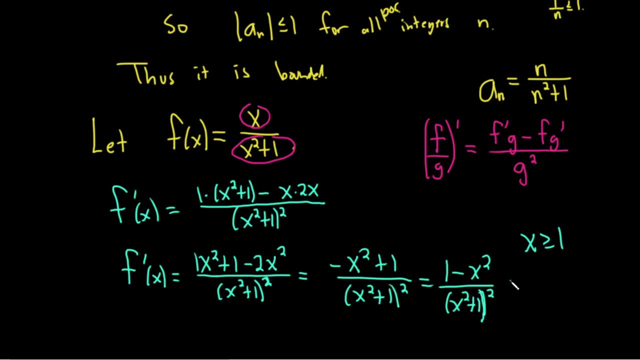 this is interesting because this here is going to be um, less than or equal to zero, because the smallest- uh rather the biggest this can be is when x is one and x is less than or equal to one. right, if x is one, you get one minus one squared, so you get zero, so the whole thing is zero. 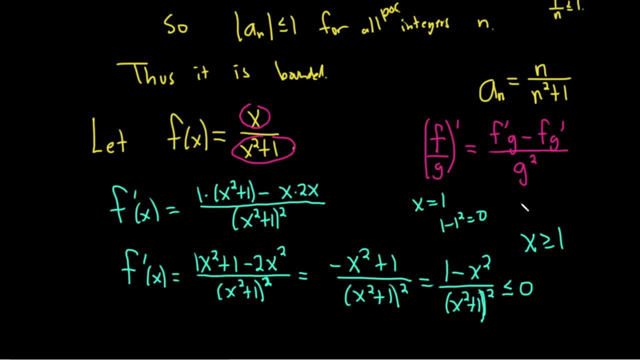 now x is an integer here, right, remember, this is going to be a sequence. so when x is two, you get that right. that's less than zero and the bottom is always positive. so this thing is going to be negative for x bigger than one. so for x bigger than one. 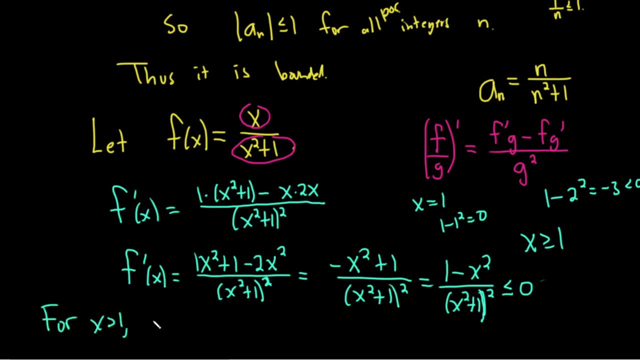 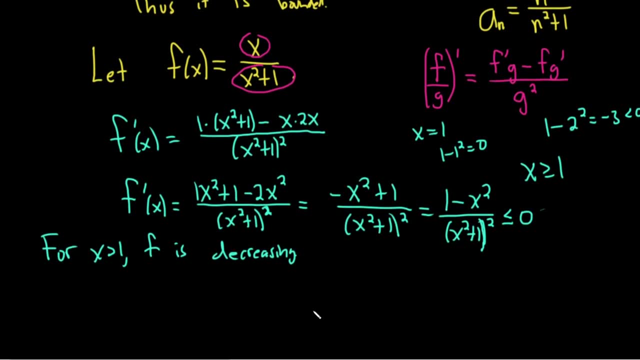 uh, f is decreasing, right. so uh, in this case our sequence is decreasing. so you just simply say a sub n is decreasing, right, because if it's decreasing for values of x- uh, bigger than one- it's certainly decreasing for integers bigger than one as well. so so it is monotonic, right, it is monotonic mono.